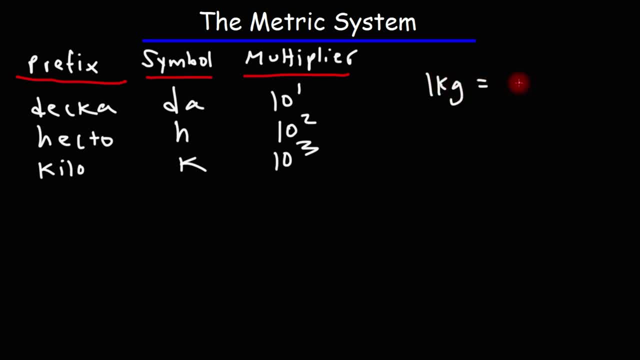 deca is a symbol for deca and it's 10 to the 1, or just 10.. One kilogram is 1,000 grams, or 1 times 10 to the 3rd grams. Next up we have mega. 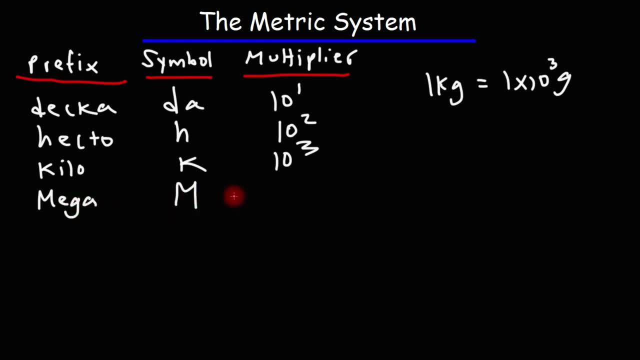 Now it's not going to be a lowercase, but this is a capital case. capital M And this is 10 to the 6th. Mega is basically a million. So a megawatt, a megawatt power plant, produces 1 times 10 to the 6th watts, or a million watts. 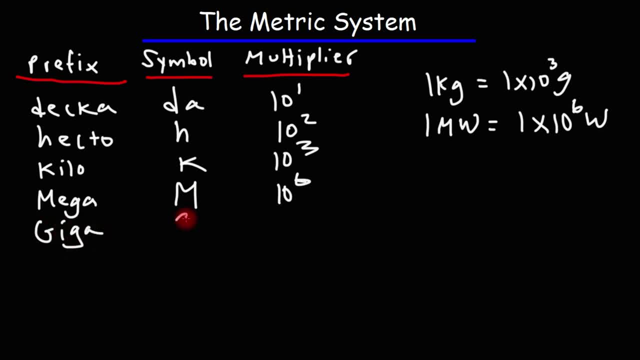 Next up we have mega. Next up we have giga, represented by the symbol capital G. Giga is 10 to the 9,, which is equivalent to a billion. So a gigajoule is 1 times 10 to the 9 joules. 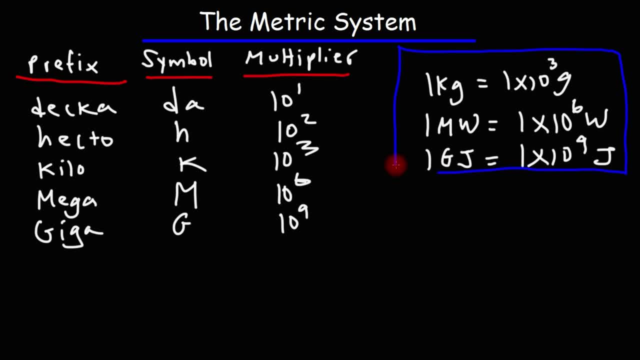 So what I have here are called conversion factors. Notice how I'm writing all of my conversion factors. This is going to be important when we're solving problems. So what you always want to do is you always want to attach a 1 to the prefix. 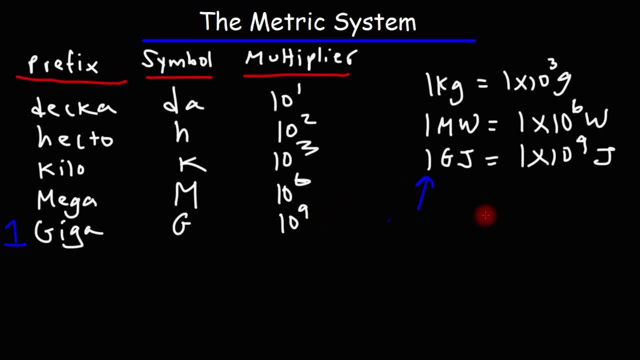 And then the multiplier goes with the base unit, whether it's joules for energy, watts for power, grams for mass. So you always attach the multiplier to the base unit And it makes it easy to write the conversion factors. Once you have the conversion factors down, then it's going to be easy to convert from one unit to another. 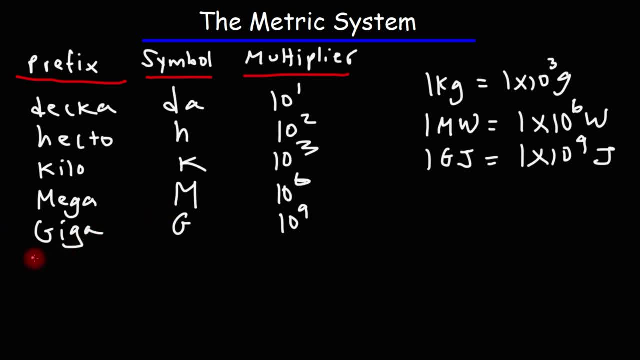 After giga, what we have next is Tera, capital T. Tera is 10 to the 12,, which is equivalent to a trillion. So 1 terawatt is 1 times 10 to the 12 watts. 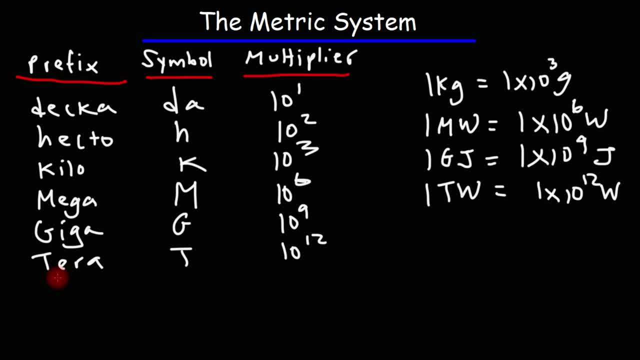 After tera, the next one in the list is peta. In most cases, if you're studying for an exam, typically you need to know up to tera. So go and pass 10 to the 12. You usually don't need to know these unless your professor gives you you know these notes. 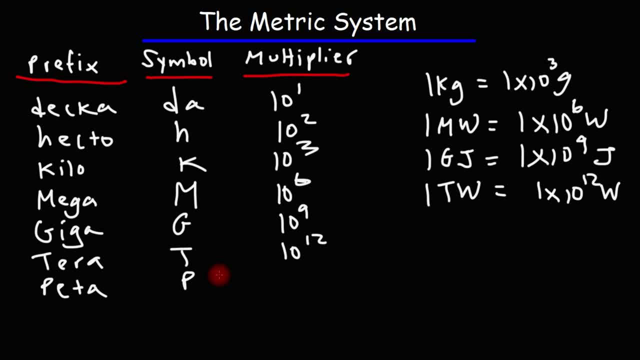 But usually up to 12 is. you know the limit, But there are some other ones beyond 12, and I'm going to give it to you. Peta is 10 to the 15.. So remember, mega is a million. 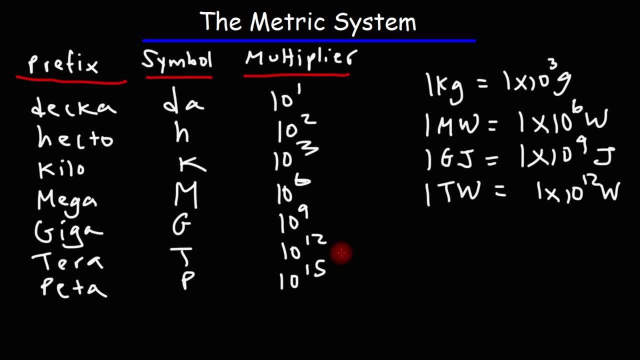 Giga is a billion, Tera is a trillion, Peta represents a quadrillion And exa capital E, that's 10 to the 18, which is a quintillion. After exa you have zeta And that's not a lowercase z, but this is a capital Z. but I am running out of space. 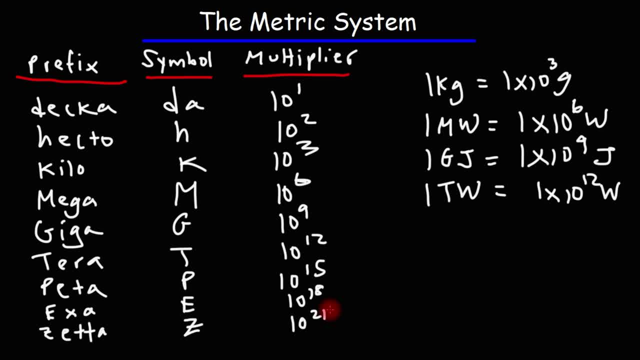 Zeta is 10 to the 21st, or 10 to the 21. And that's 10 to the 21st, That is a sextillion. After that we have yoda, represented by the symbol capital Y. 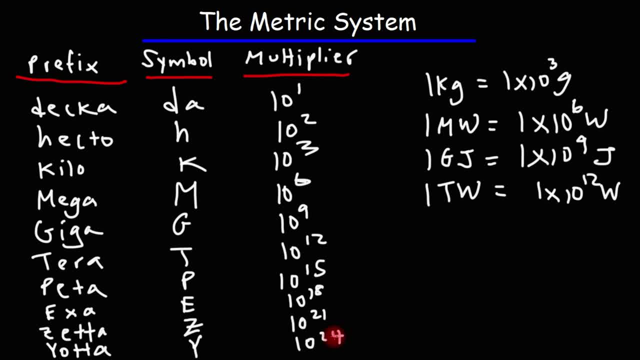 And that's 10 to the 24th, which is a septillion. So if you know up to 10 to the 12th, you should be okay for your exam. Now let's go over the multipliers that have a negative exponent. 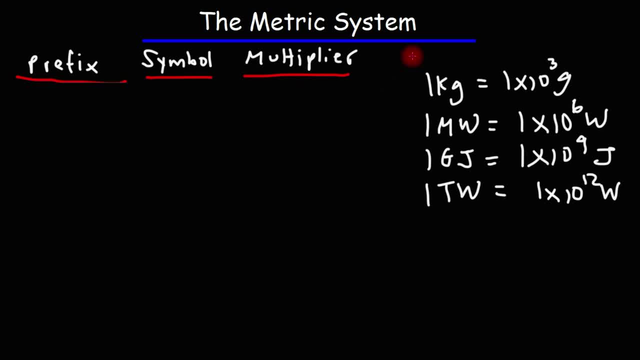 This is the other half, So let's start with the prefix deci, represented by the symbol lowercase d. Deci is 10 to the minus 1.. Next we have centi, lowercase c, That's 10 to negative 2.. 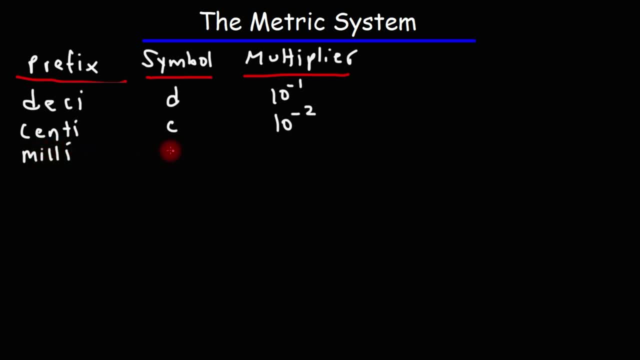 And then milli lowercase m is 10 to the minus 3.. the only time you have a capital symbol is mega and above, like mega, giga terra and anything above that. everything else the symbols are lowercase. so think about what this means, think about how. 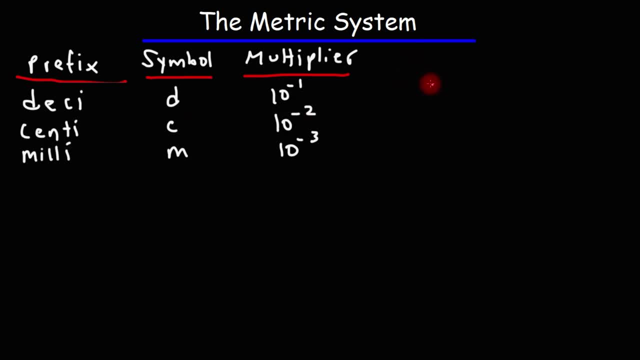 we can write a conversion factor with this information: one centimeter: always put a prefix in front of, put a one in front of the prefix. one centimeter is one times ten to the minus two meters. so always attach the multiplier to the base unit. one milliliter is one times ten to the minus. 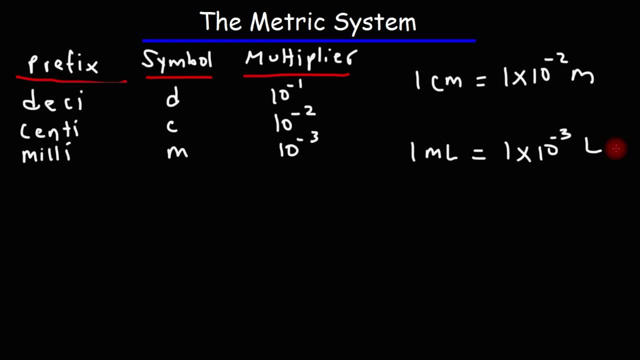 three liters. now, once you write this conversion factor, what you can do is you can alter it. if we multiply both sides by a hundred, we get that a hundred centimeters is equal to one meter. ten to negative two is equal to one meter. so if we multiply both sides by a hundred, we get that. 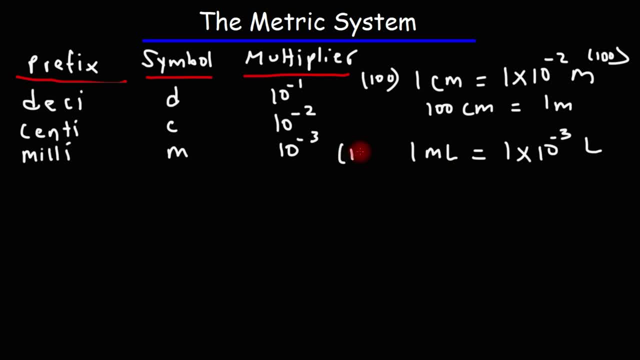 times a hundred is simply one. if we multiply this by a thousand, we'll get this common conversion factor. a thousand milliliters is equal to one liter, so if you can write the standard conversion factors, you can get the common ones as well, simply by adjusting the equation. 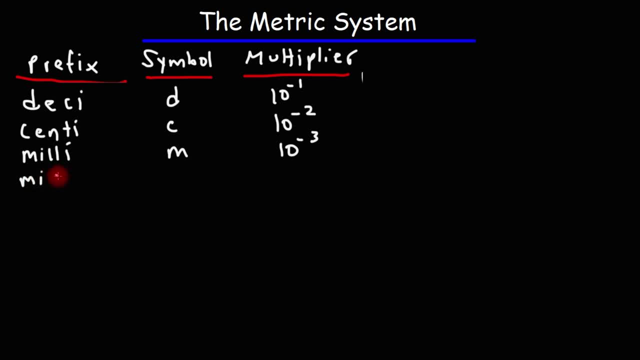 now, after milli, the next one is micro. micro is ten to the minus six, so one micrometer is one times ten to negative six meters. after micro, we have a nano, lowercase n. nano is ten to the minus nine, so think of ten to the nine, which was giga. that represents one billion nano. ten to negative nine. 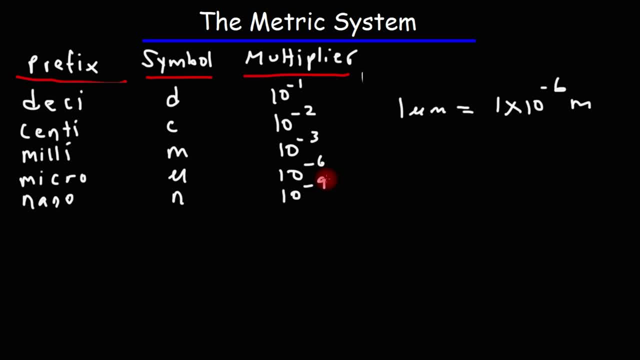 is a billionth. mega ten to the six was a million. micro ten to the minus six is a millionth, with a th at the end. so one nanometer is one times ten to negative nine meters. after nano it's pico, lowercase p. ten to negative twelve: one picometer. 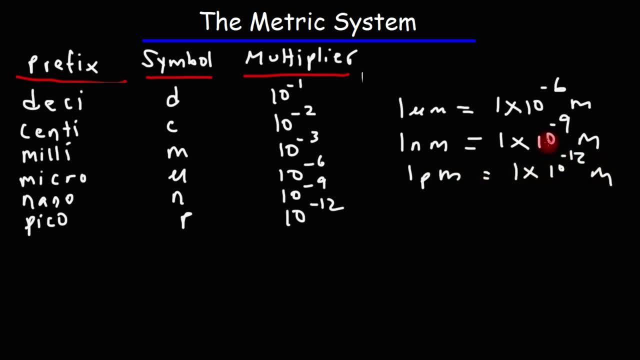 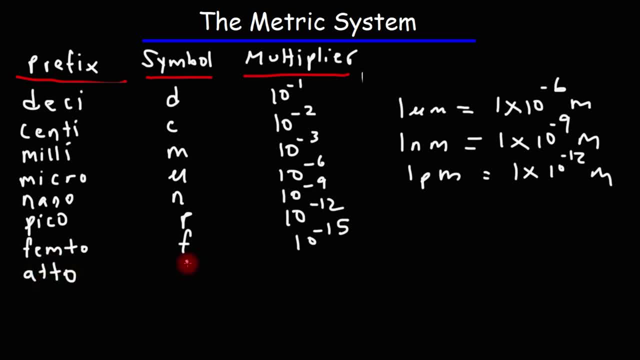 after femto is addo with the symbol, lowercase a, and this is 10 to negative 18.. after addo it's zepto, lowercase z: 10 to negative 21, and after zepto it is yakdo, lowercase y, 10 to negative 24.. 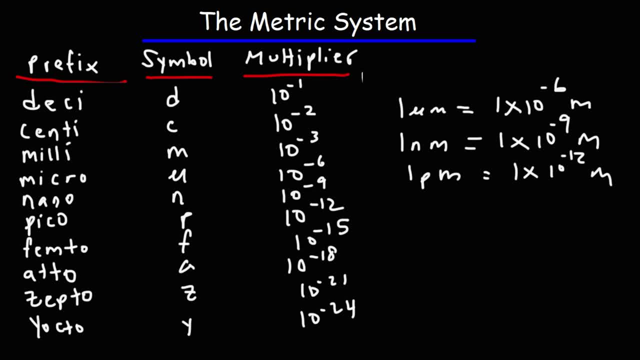 but for the smaller units, typically you need to know up to pico. so you need to know from pico 10 to negative 12 to tera 10 to the positive 12.. those are the common prefixes that you're going to encounter in class. the other ones, they're optional, typically they're not commonly used. 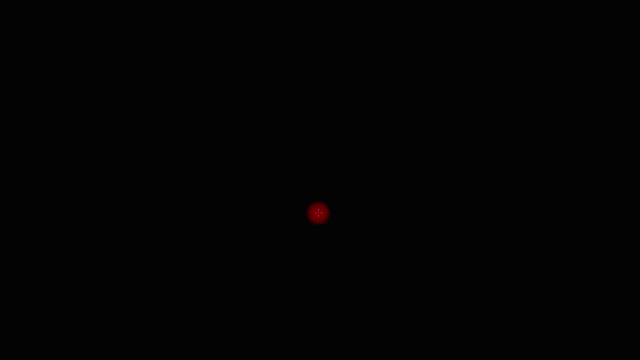 now let's talk about how we can convert from one unit to another. so, for instance, let's say, if we have 478 meters and we wish to convert it to kilometers, how can we do that? well, this is a one-step conversion problem, so we just need to know the conversion factor between kilometers and meters. 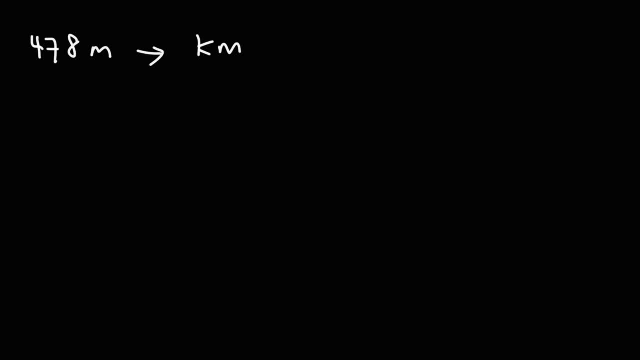 we know that kilo represents 10 to the third, or a thousand, so we can write the conversion factor one kilometer. i always put away 1.4 kilometers, so we can write a conversion factor one kilometer. always put away one kilometer, one in front of the prefix. One kilometer is one times ten to the third meters. So step one. 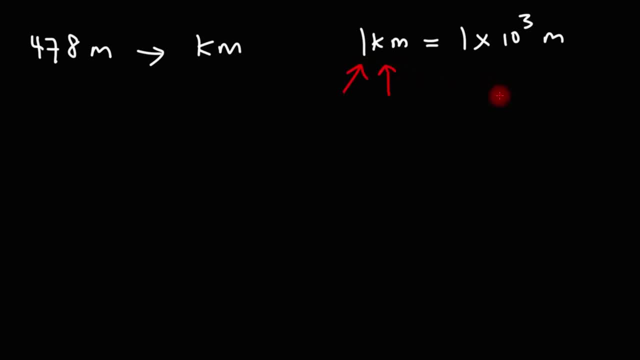 write a one, write the prefix with the base unit, write the multiplier and then the base unit without the prefix. And that's how you can write your conversion factor. Now, to convert it, start with what you're given. We're given 478 meters. We'll put it over one. 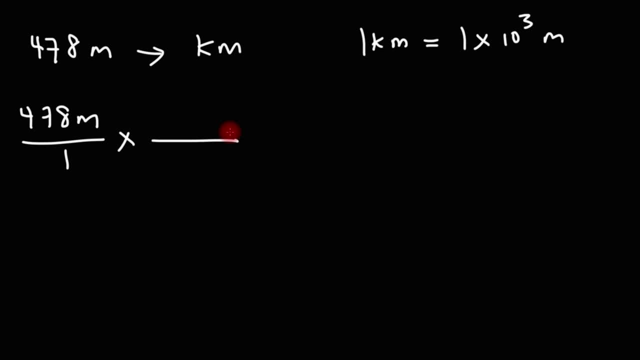 In the next fraction we're going to put our conversion factor. Notice that we have the unit meters on top. So to cancel meters we need to put this part of the equation in the bottom. This is going to be one times ten to the three meters and then the other part is going to go on. 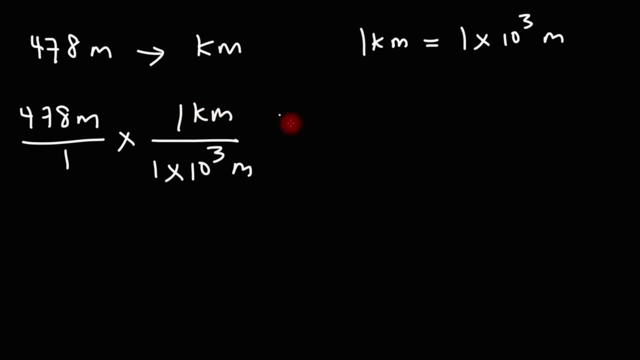 top. So we need to set the fractions in such a way that the unit we want to convert from this expression is going to be one times ten to the three meters And the unit that we want to get to remains. So this becomes 478 divided by 1,000,. 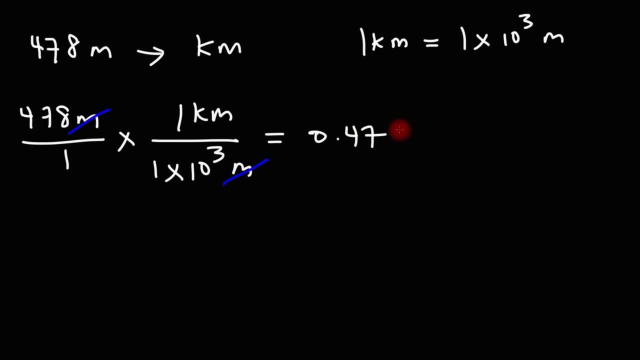 and that gives us the answer 0.478 kilometers. So that's how you can do a one-step conversion problem. Let's try another one. Let's say we have 400, actually let's say 0.236 liters, and we want to convert that to milliliters. 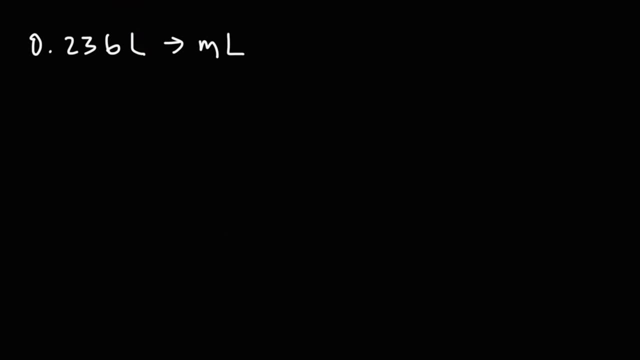 Feel free to pause the video and try that example. So first let's write the conversion factor. One milliliter is equal, to remember it's ten to the minus three, so it's going to be one. and then we're going to put the multiplier. 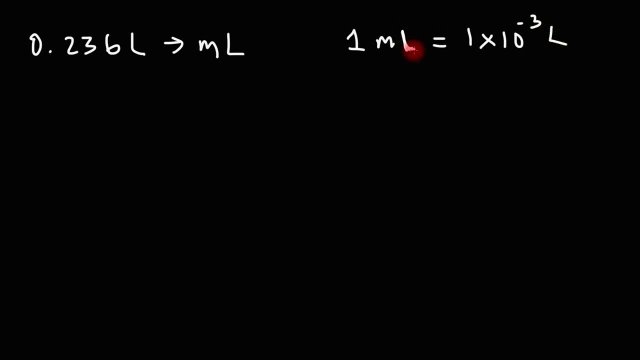 ten to negative three, and then the base unit liters. So that's our conversion factor. Now let's start with what we're given. We're given 0.236 liters. We'll put that over one. Now we got to find out what goes on the top and the bottom of. 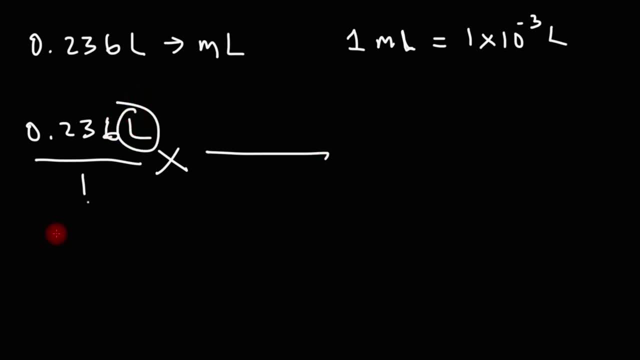 the next fraction. Since we have liters on top of the first fraction, we want liters to be on the bottom of the second, Which means milliliters have to go on top. So this number attached to liters has to go on the bottom. 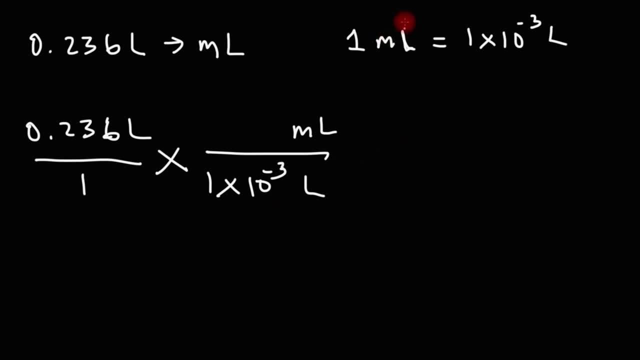 So we'll put one times ten to the minus three liters on the bottom, and then this will by default go on top. So this tells us that we need to divide by a thousand to convert liters into milliliters. Actually, not by a thousand, We need to divide by 10 to the minus three liters. 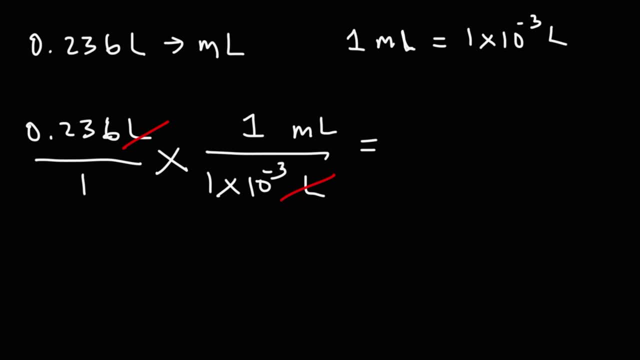 which is 0.001. that has the equivalent effect of multiplying by a thousand, so it's 0.236. you can divide it by 0.01, or if you multiply by a thousand, you're going to get two hundred and thirty six milliliters. by the way, when dividing this, put this in parentheses because your 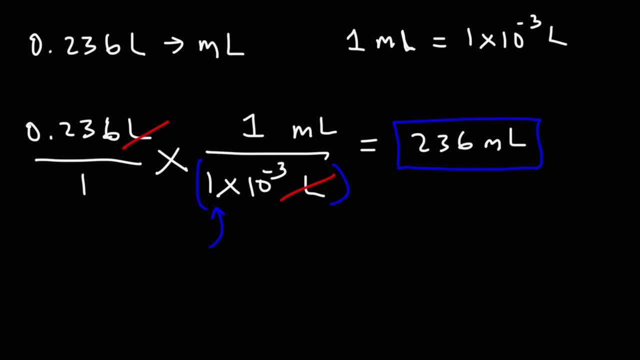 calculator may divide by 1 and then multiply by 10 to negative 3. now let's try a two-step conversion problem. let's say we have 496 micrometers. we want to convert that to actually. let's say, this is in picometers, 496 picometers, and we want to convert that to. 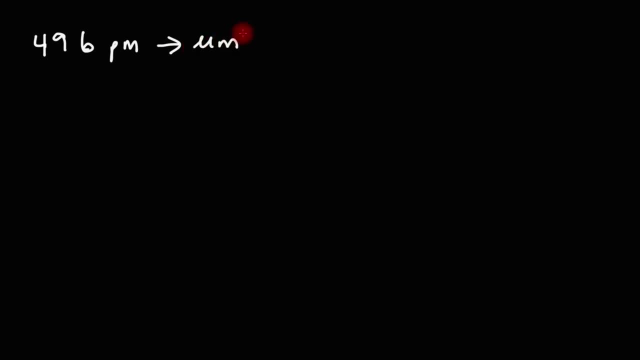 micrometers. try that problem now, even though there are shortcut methods available that you can use. what I'm going to do is I'm going to do this one step at a time. I'm going to convert picometers into the base unit meters, and then meters to micrometers. 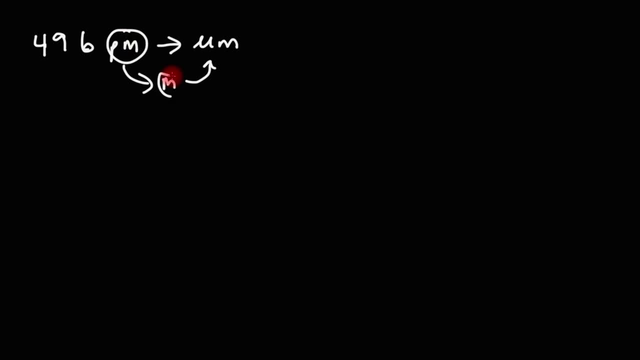 so let's write the conversion factor from picot to meters. picot is 10 to the minus 12, so 1 picometer is 1 times 10 to negative 12 meters. we'll use that in the first step. for the second step we'll. 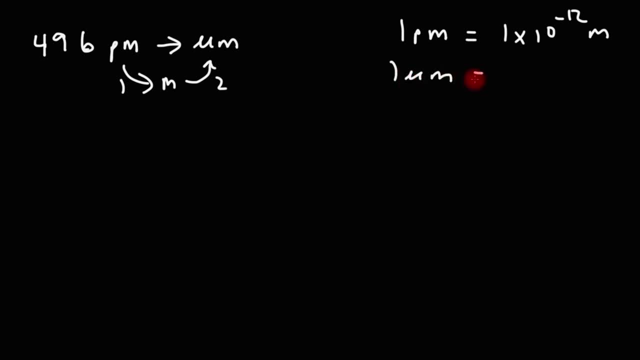 convert meters to micrometers. 1 micrometer- we know it's micro- is 10 to the minus 6, so it's 1 times 10 to negative 6, and then the base unit meters. so let's start with what we're given 4. 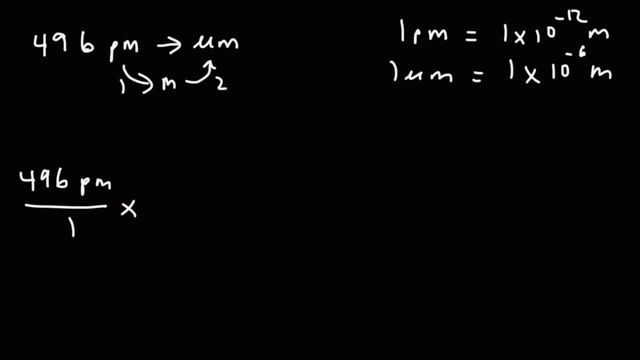 6 picometers over 1. let's use the first conversion factor to go from picometers to meters. so because we have the unit picometers on the top left, we're going to put it on the bottom right of the second fraction. meters is going to go on top. so we have: 1 picometer is equal to 10 to negative 12 meters. 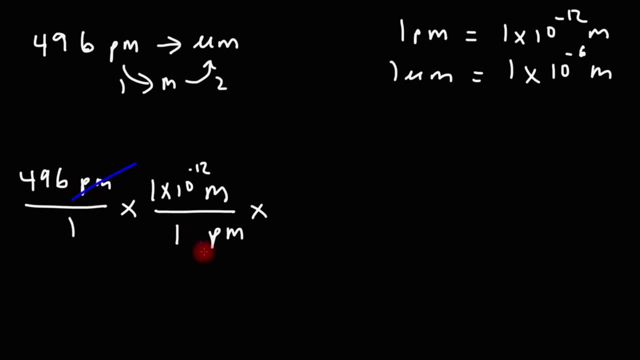 so now the unit picometers will cancel. and now let's use the second conversion factor to go from meters to micrometers. since we have meters here, we're going to put meters on the bottom, micrometers on top, so it's 1 micrometer and the number that's attached to meters is 10 to negative. 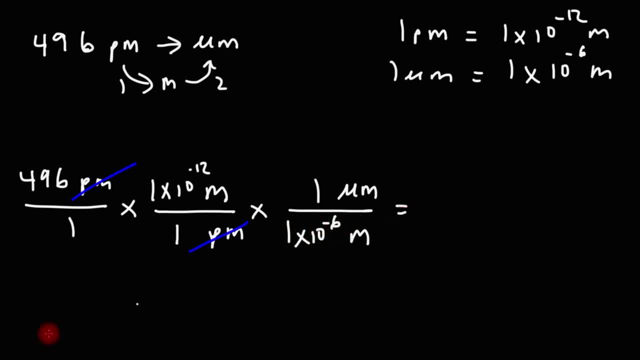 6. so now we can cross out the unit meters. so when we do the math we're going to have: 1 picometer is equal to 10 to the minus 6. so we're going to get the answer so you can plug this in your calculator. 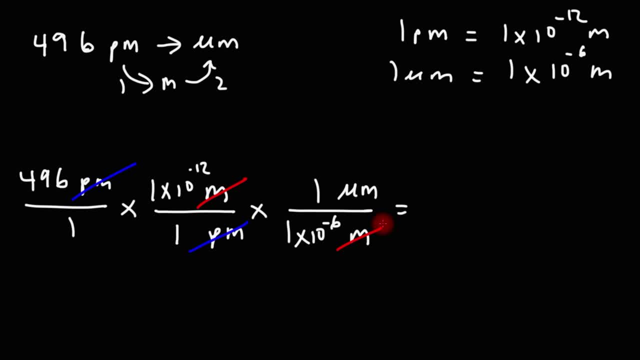 or you can do it mentally. let's talk about how we can do this mentally. so we have 496. we can ignore the one. what's important here is the 10 to negative 12. now notice that we have a 10 to negative 6 on the bottom. what we can do is take this and move it to the bottom, and then we can. 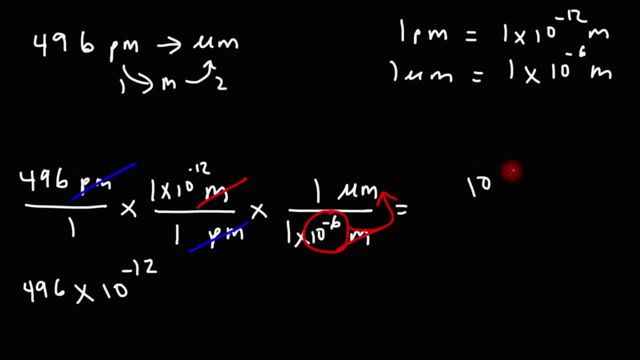 move it to the top. if you have, let's say, x to the negative 3, this is 1 over x cubed. if you move it from the bot, from the top to the bottom, the exponent changes sign. it goes from negative 3 to positive 3.. likewise, if you have a negative exponent on the bottom and you decide to move, 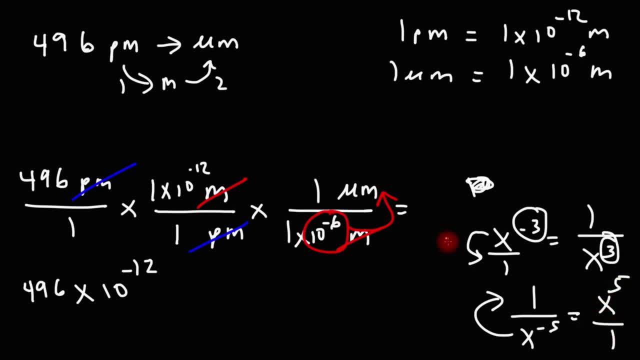 it to the top, it'll go from negative to positive. so if you flip it or if you move it from one side to the other side of the fraction, it's going to change sign. so it's 10 to negative 6 on the bottom, but when we move it to the top it's going to be 10 to 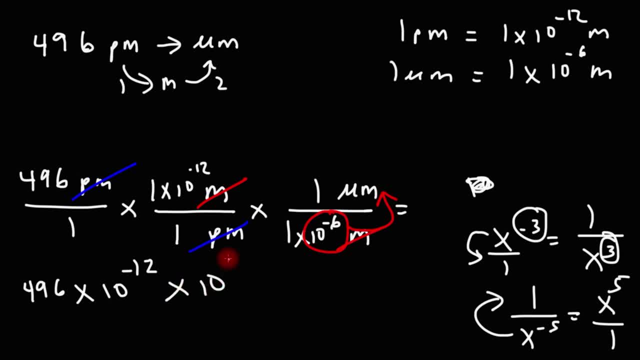 the positive 6.. now, when multiplying common bases, we can add the exponents negative 6, I mean negative 12 plus 6. that's going to be negative 6.. so we have 496 times 10 to negative 6 and the unit is: 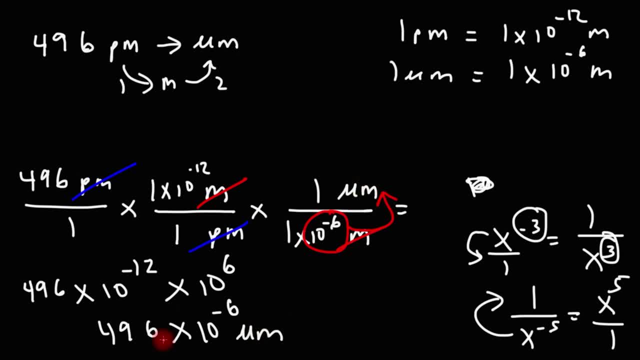 the unit that's left over micrometers. now we need to move the decimal two units to the left. 496 is the same as 4.96 times 10. to the second: power: 10 squared is 100, so 4.96 times 100 is 496. and then we still have 10 to negative 6 as well. so 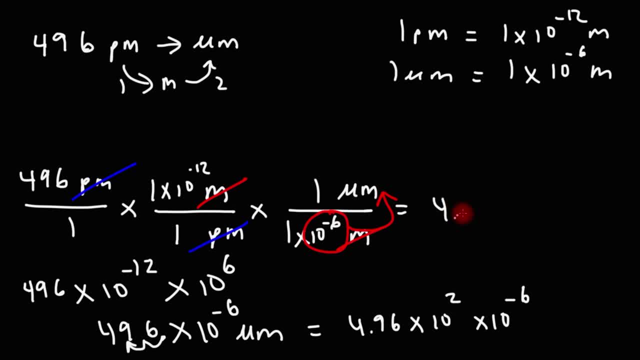 adding these two will give us negative 4. the final answer is going to be 4.96 times 10 to the negative 4 micrometers. so that's how you can do a problem like that without the use of a calculator. we typically leave our answer in scientific notation, so you want the decimal. 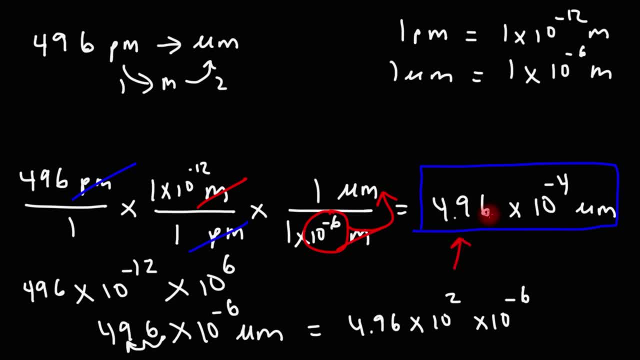 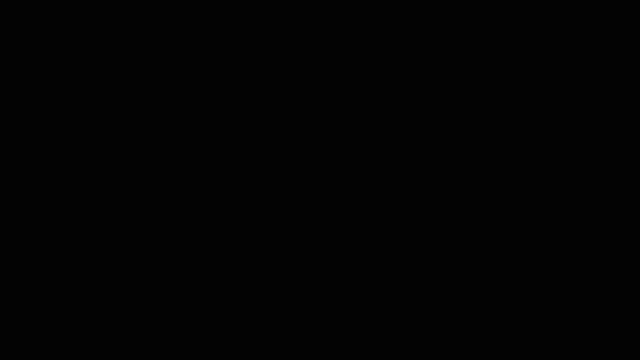 point to be between the first two non-zero numbers. now let's try another example. let's say we have 3.54 times 10 to the negative. actually was a positive 10 to the positive 7 nanometers, unless convert that to kilometers. go ahead and try that problem. by the way, for those of you who want, 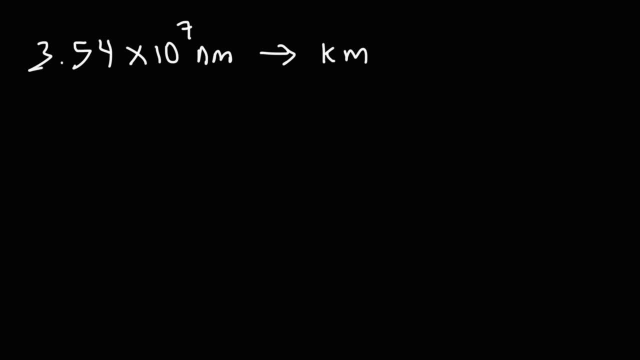 harder problems to work on. go to the YouTube search bar. type in unit conversion, organic chemistry tutor and a video that I've created- it's a very long video- will show up and you'll get more harder problems that involve unit conversion. now for this problem. what I'm gonna do is I'm gonna convert nanometers.